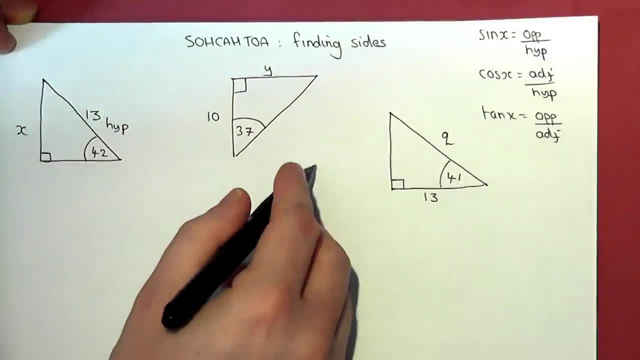 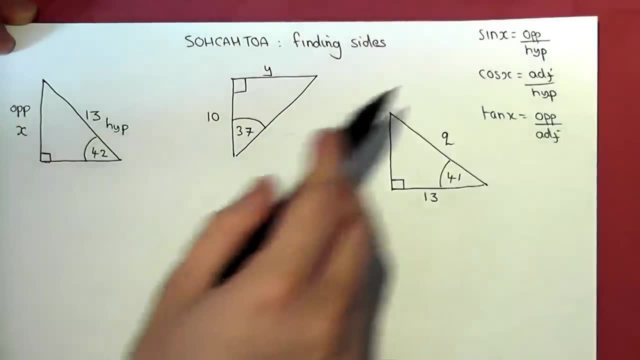 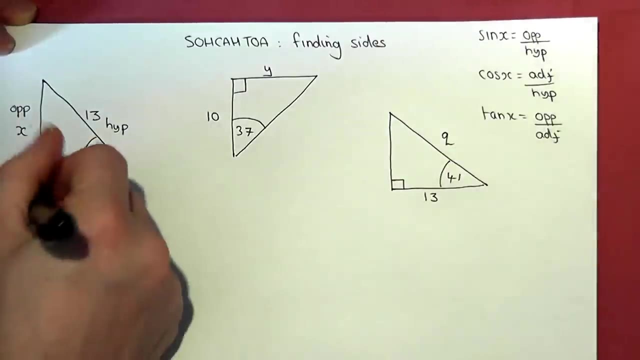 it's opposite the right angle. But the unknown is opposite the angle. so that's called the opposite And we then identify which of the equations uses opposite and hypotenuse. Well, it's the sine equation, So sine. now, the x here in the equation is the angle, not the 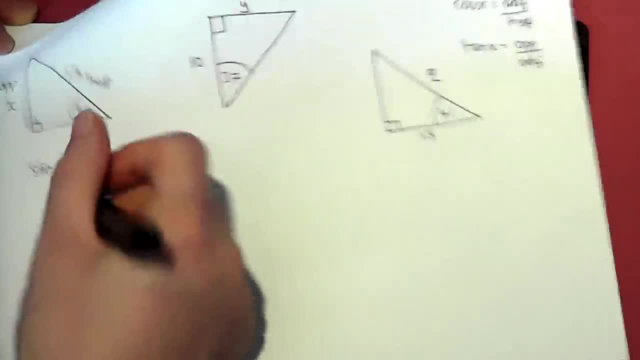 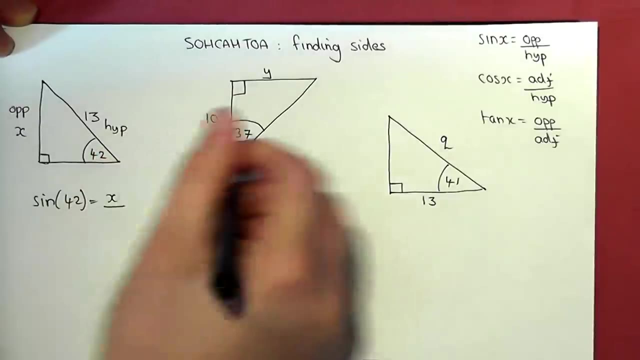 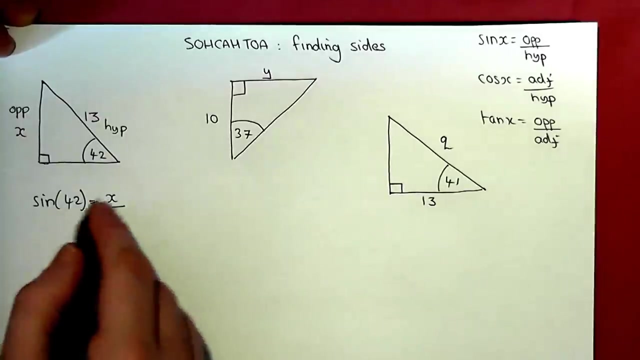 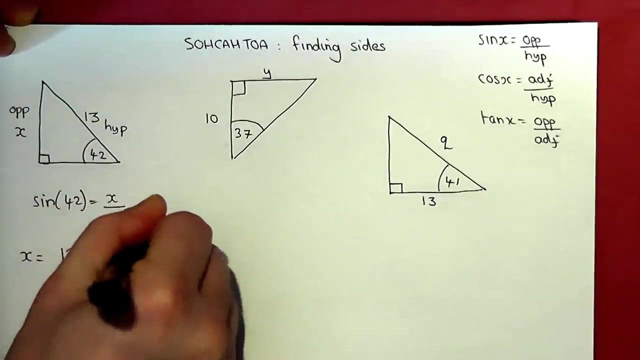 x in the equation. So sine of the angle, in this case 42, is equal to opposite, which is x over the hypotenuse, which is 13.. So to find x I need to rearrange this equation by timesing by 13.. So x equals 13 lots of sine 42. So I input that into my 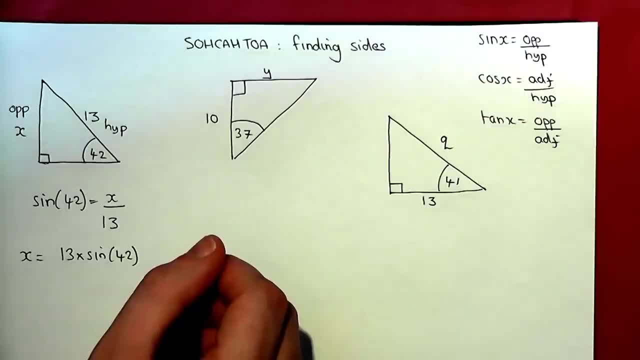 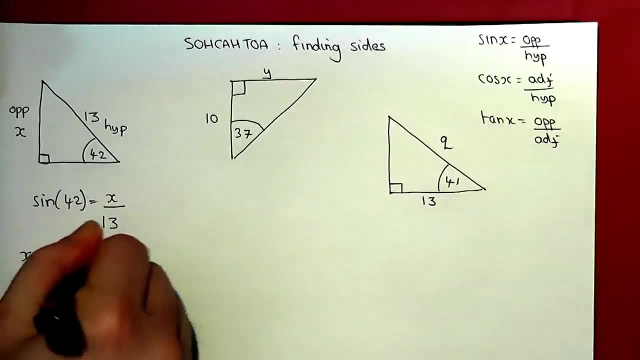 calculator, as I see it, 13 times sine of 42. And I get 8.7.. Subtitles by the Amaraorg community. I hope this video was more informative and helpful. We'll see you then. Subtitles by the Amaraorg community. 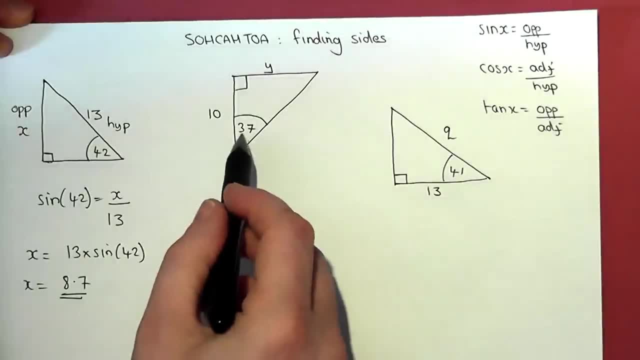 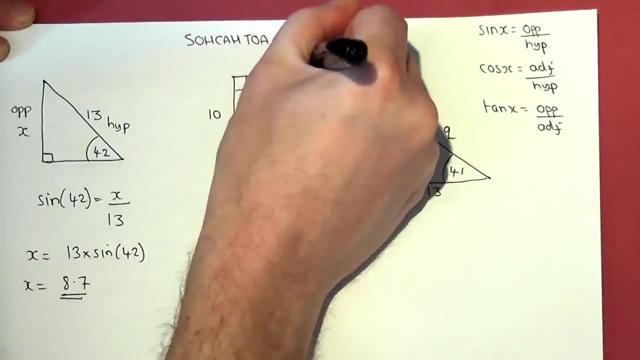 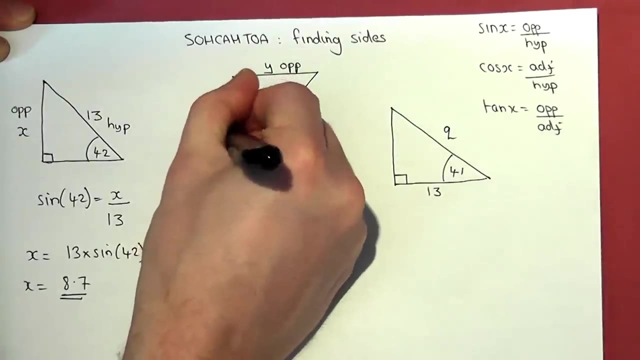 ok, so we also have a number where we have two numbers here and that value we need to apply to the suppose Y. We really just think that we have to use a procedure to put two zeros equal to two zeros For that first one. of course we need to answer the question: why was the triangle adjusted? 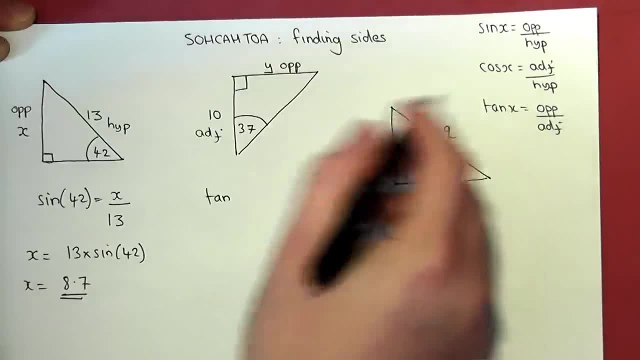 to the angle. The argument we would get is that when x is warfare, according to the set of numbers, Z equals 1 minus z minus z minus z equals 32.. And, as I have said, even if I think that like a circle, perhaps tua� means a dash, whatever, 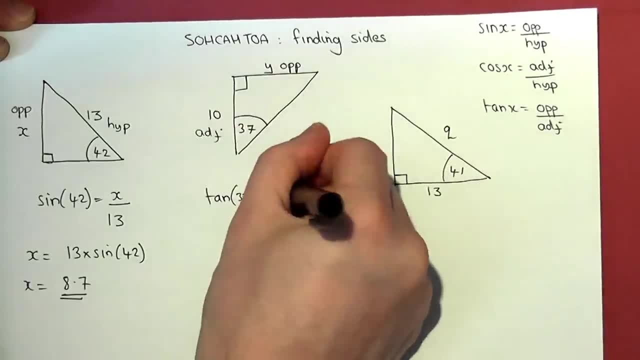 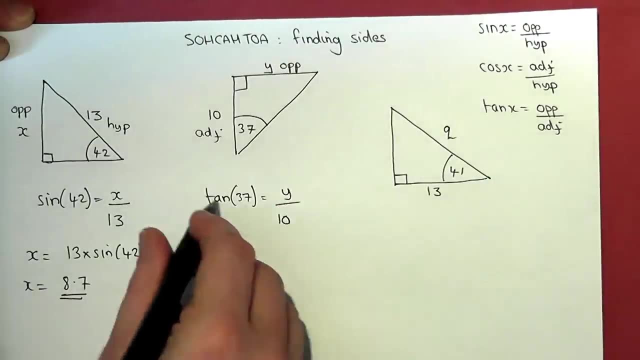 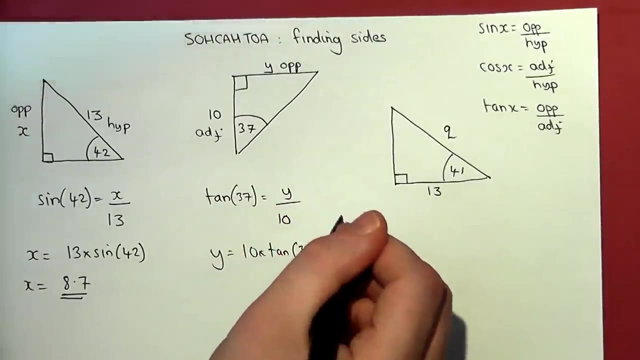 so the angle equals opposite y over the adjacent. So again, to find y I must rearrange the equation by timesing by 10.. So y is 10, lots of tan 37. So I input that into my calculator: 10 lots of tan of 37, and the answer is 7.5.. So y has a length of. 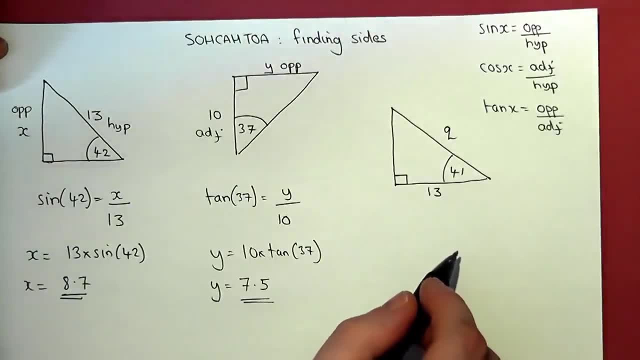 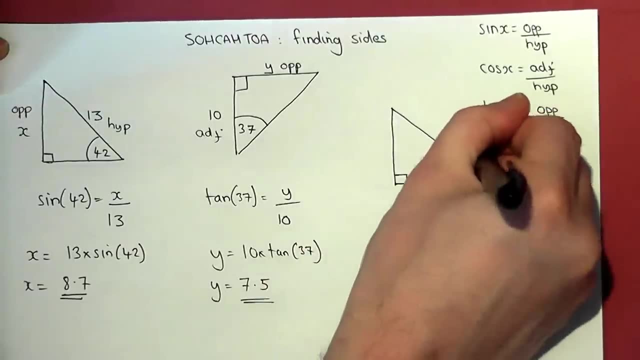 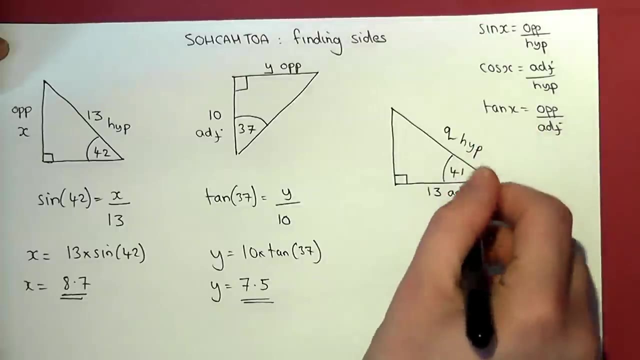 7.5.. Now then the third one Angle, known, unknown. The unknown is opposite the right angle, That is the hypotenuse. This side here is next to the angle, It is the adjacent. So adjacent hypotenuse is cos, So cos of the angle, which is 41 in this. 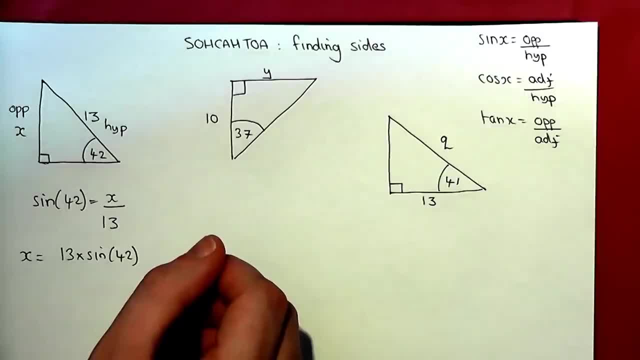 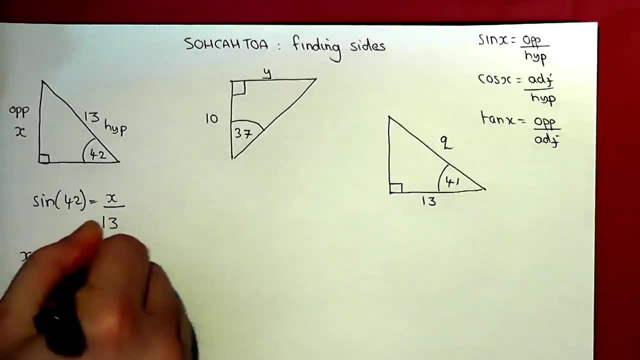 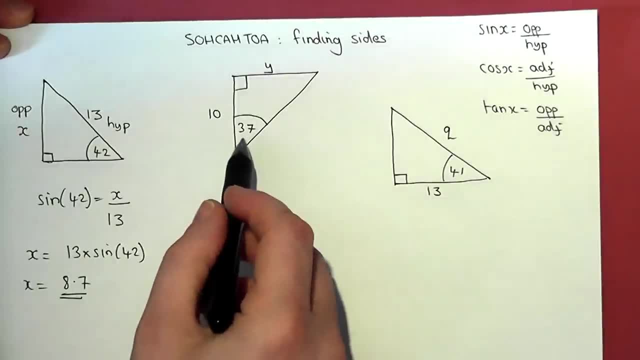 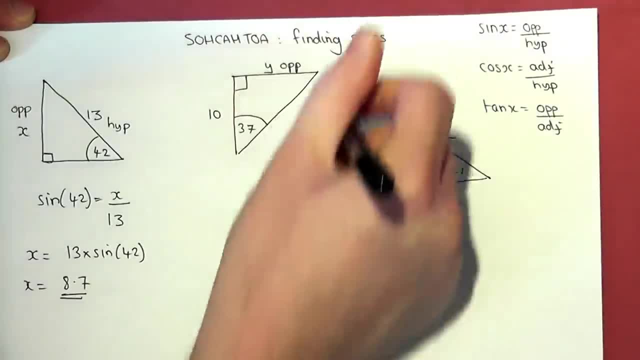 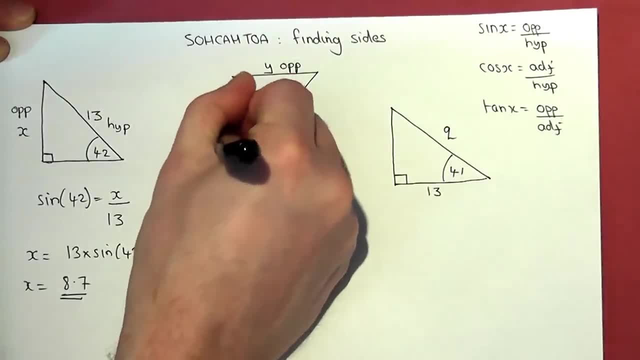 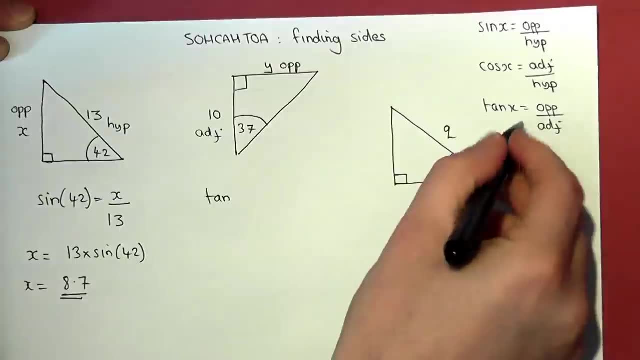 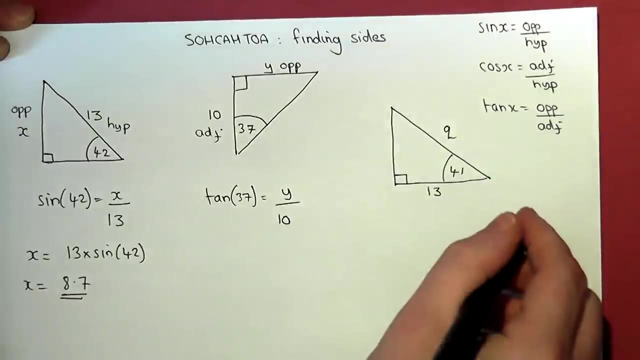 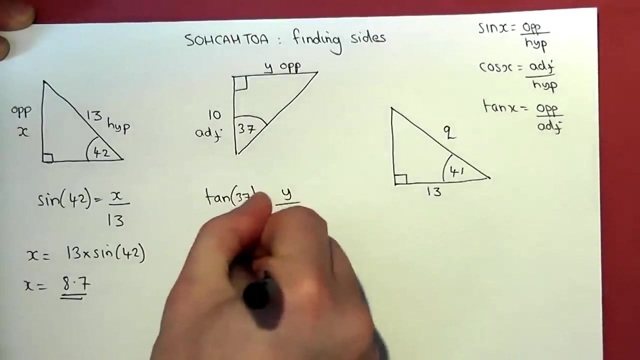 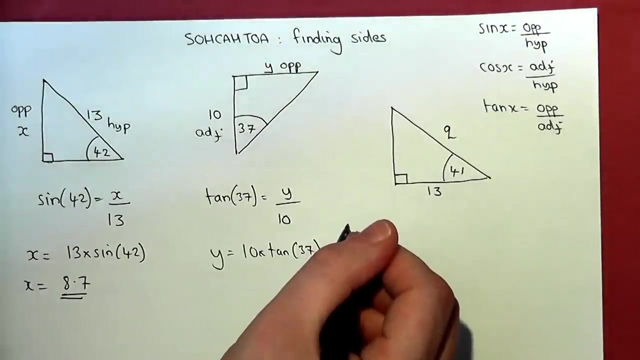 Subtitles by the Amaraorg community. it is the adjacent. So again adjacent opposite is tan. So tan of the angle 37 equals opposite y over the adjacent. So again, to find y I must rearrange the equation by timesing by 10.. So y is 10, lots of tan 37. So I input that into my. 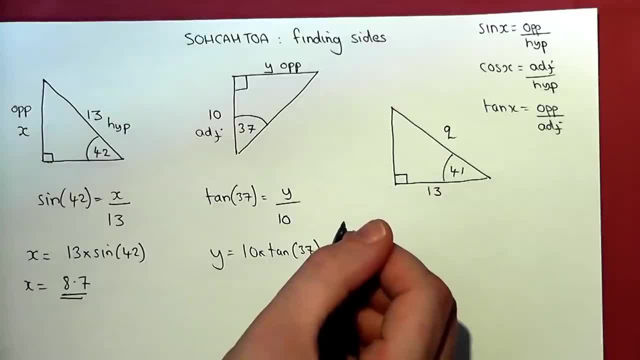 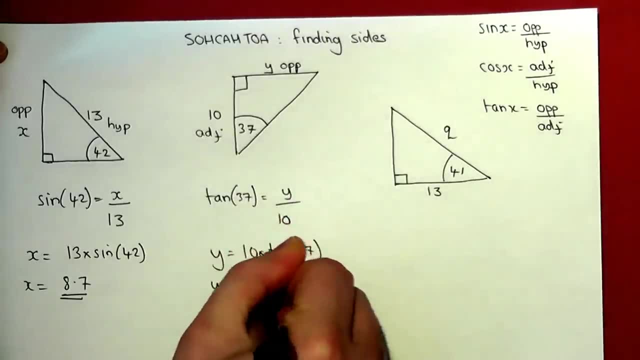 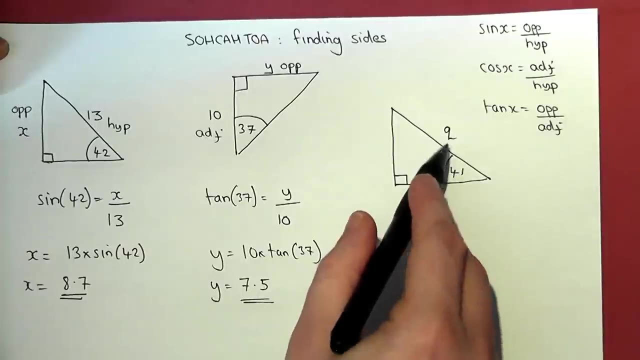 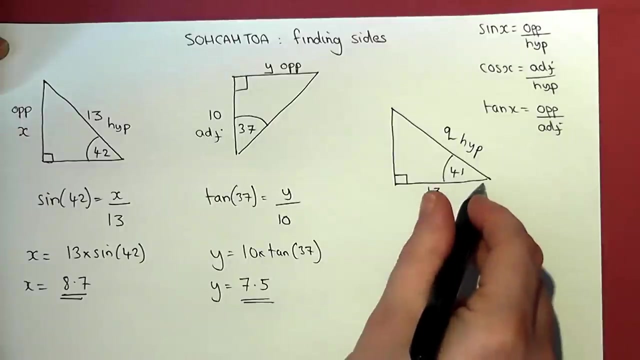 calculator: 10 lots of tan of 37, and the answer is 7.5.. So y has a length of 7.5.. Now then the third one Angle: known, unknown. The unknown is opposite the right angle, That is the hypotenuse. This side here is next to the. 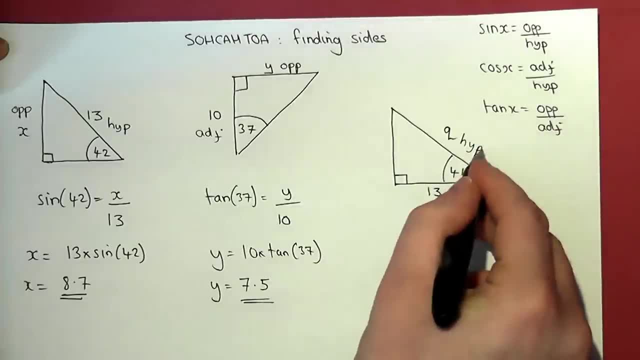 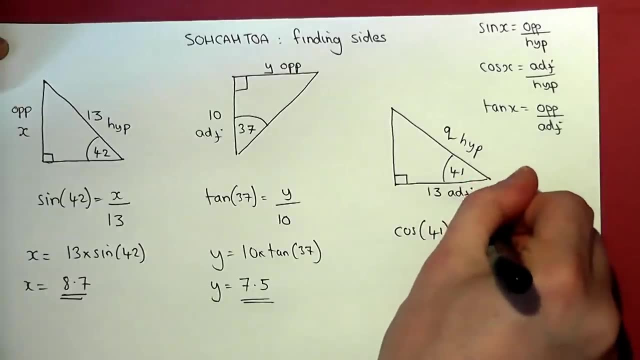 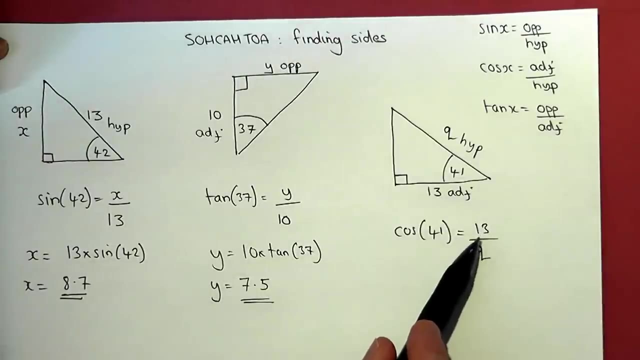 angle, It is the adjacent, So adjacent hypotenuse is cos. So cos of the angle, which is 41 in this case, is the adjacent 13 over Q, which is the hypotenuse. Now then, this is a bit different to the first two equations, because the unknown 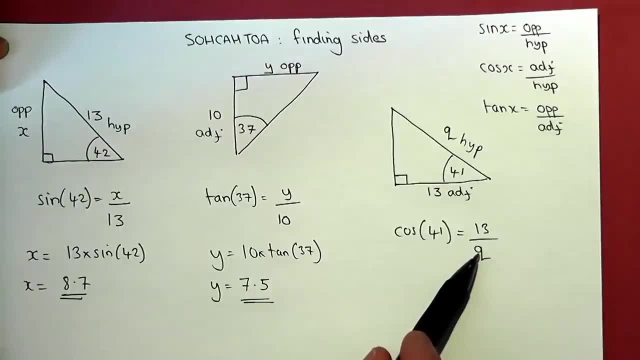 is now below the equation. So to rearrange this requires two steps. So to rearrange this requires two steps. So to rearrange this requires two steps. I first of all times up by Q, So Q, lots of cos 41 is equal to 13.. I have times by. 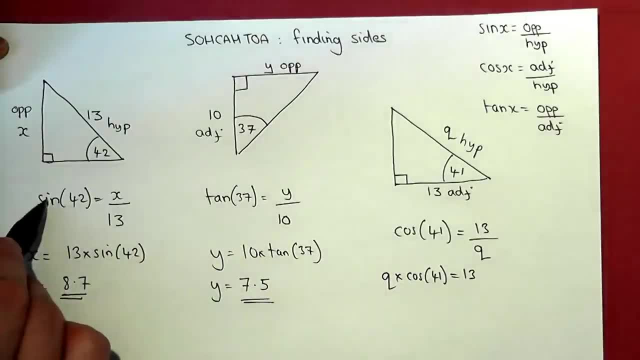 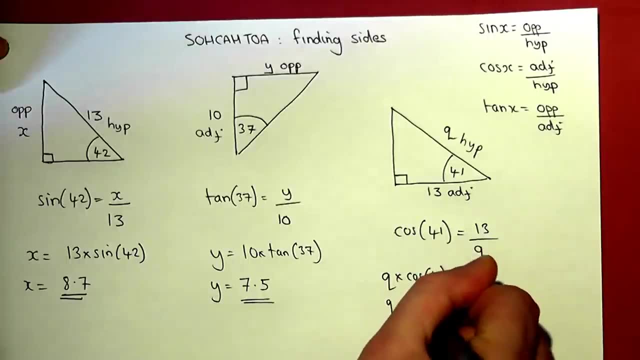 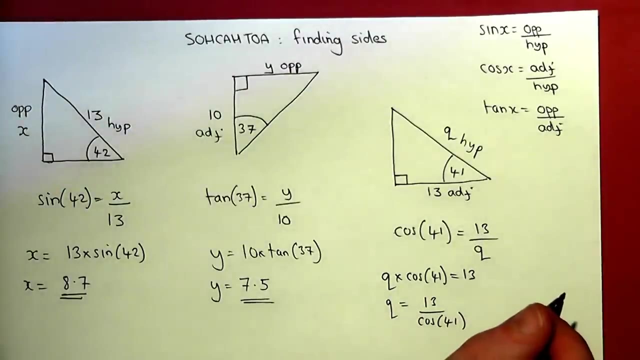 Q like I times by 10 and 13 here. So to find Q I now divide by cos of 41. So Q is 13 divided by cos of 41. So I input that into my calculator. So 13 divided by cos of 41.. 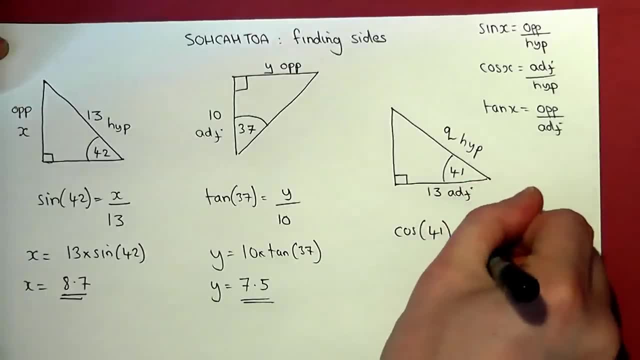 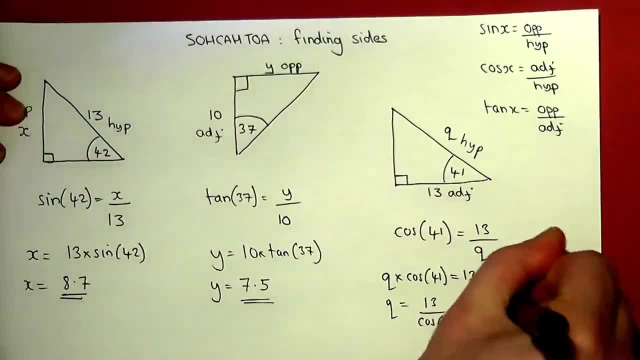 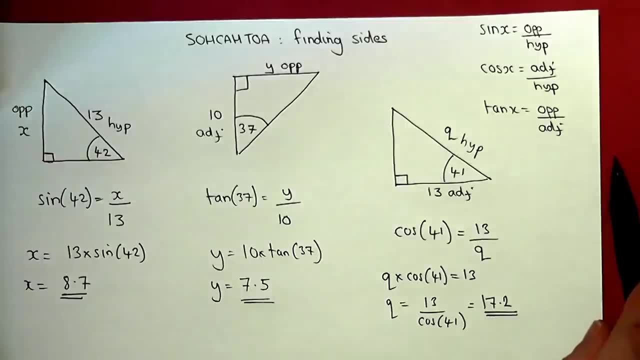 So I input that into my calculator. So 13 divided by cos of 41. And I get 17.2.. So Q has a length of 17.2.. The skills are to identify the two sides in the question, to write down the. 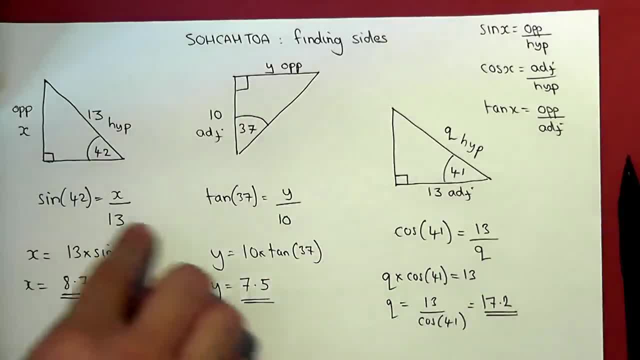 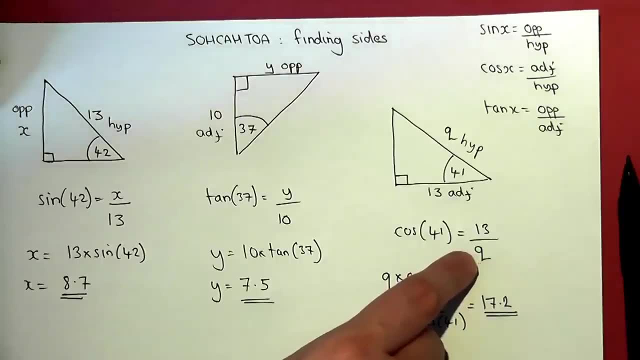 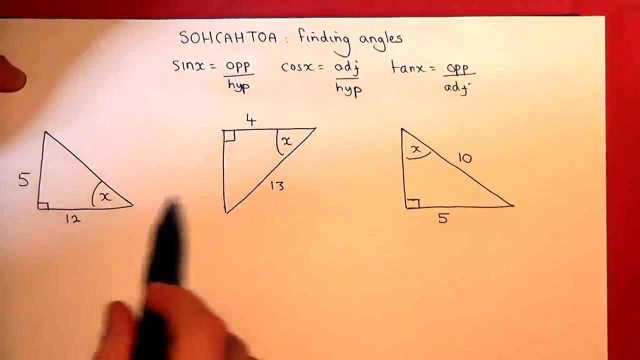 equation and then to solve it, either using the one step method, when we want the known on top of the equation, or the two step method, when the unknown is beneath the equation, That is, SOH, CAH, TOA. finding sides: This video talks through how to find missing angles when you know two sides. 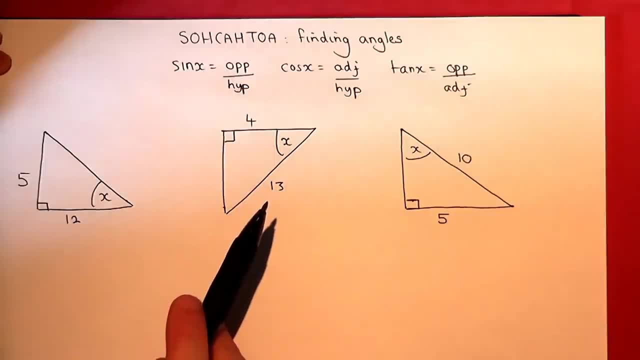 Now, then the first step is to label the sides, either opposite, adjacent or hypotenuse. Now the hypotenuse is always the longest side opposite the right angle. So hypotenuse, hypotenuse, hypotenuse From the first triangle, that's not given. But we give them the side opposite the angle. 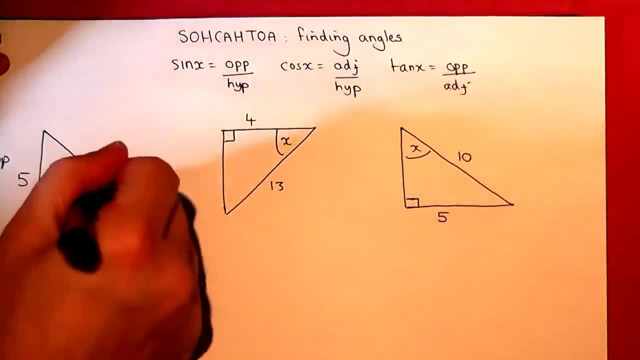 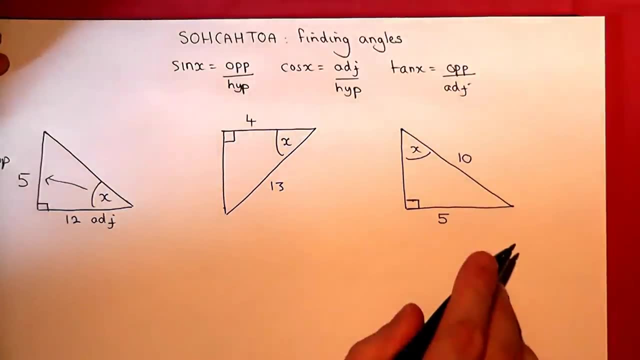 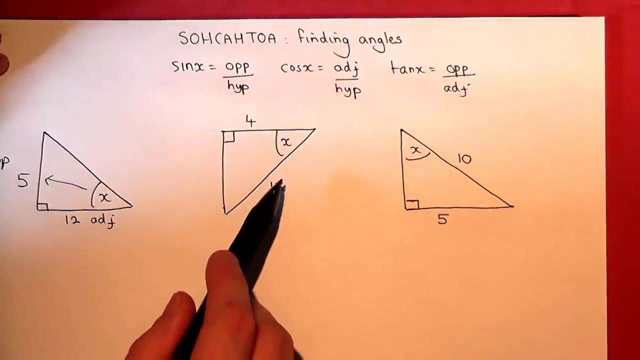 So that's the opposite. And we know the other side, which is next to the angle, That's called the adjacent Right then We then identify which of the SOH, CAH, TOA equations to use. Now we know the opposite and the adjacent, So we use the TAM equation. 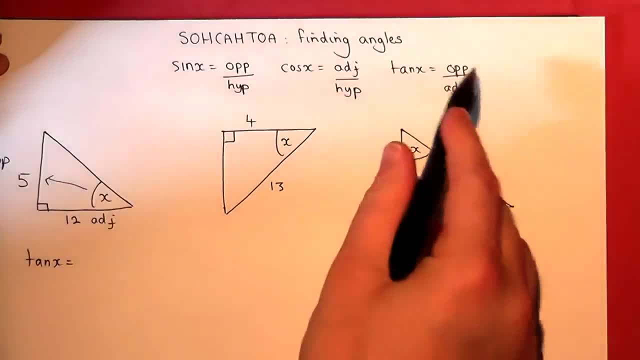 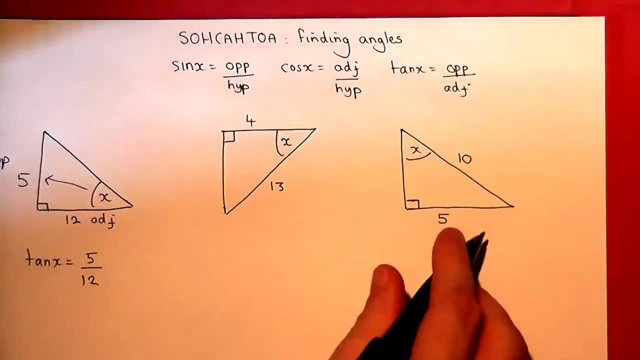 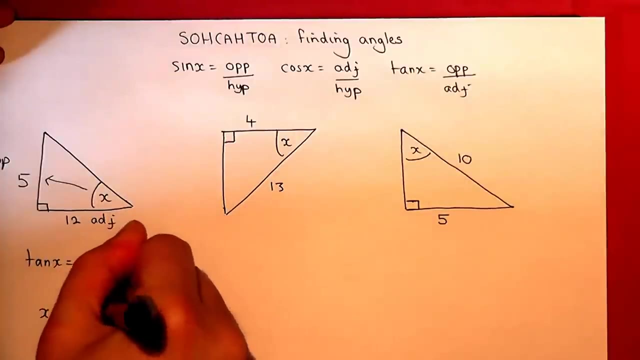 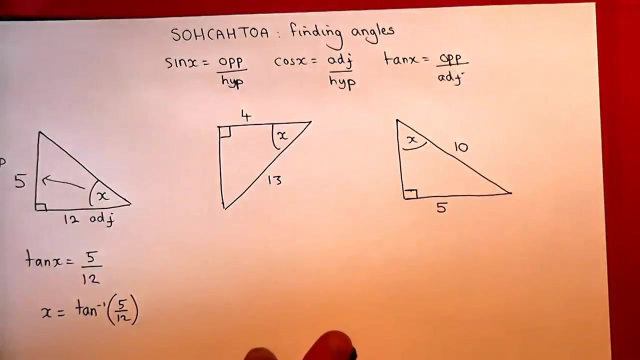 So TAM of x is equal to opposite over adjacent, Opposite over adjacent, Or 5 twelfths. Then to find out x we have to do the inverse tangent function, Or shift TAM on the calculator Or inverse TAM. So it's inverse TAM of 5 twelfths. So we put that into our calculator. 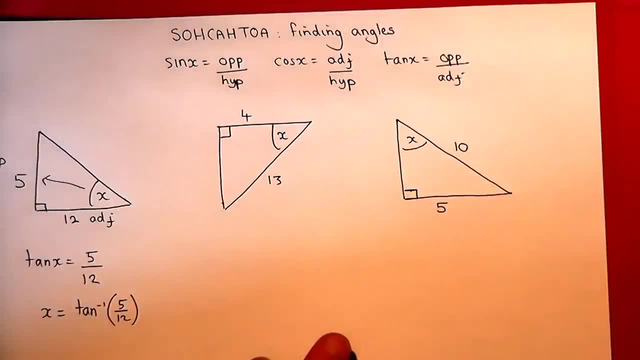 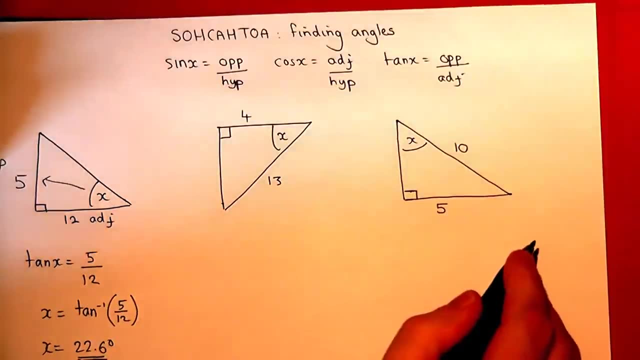 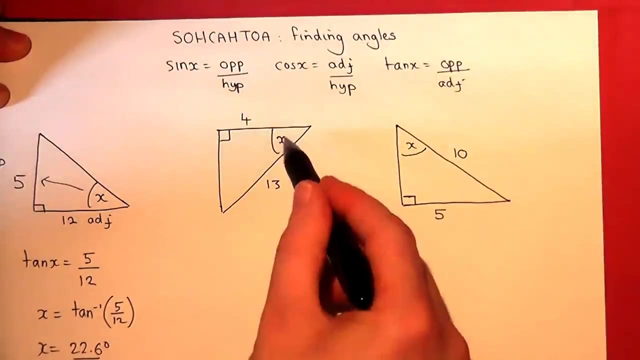 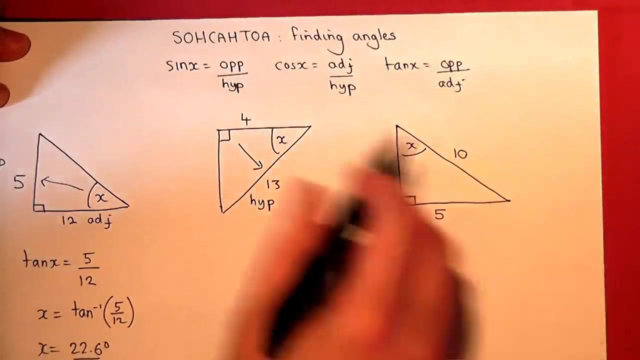 And we can do that And we get the answer, which is 22.6 degrees. The second question: We know two different sides. Here's our angle. One of them is the hypotenuse, Because it's opposite the right angle.